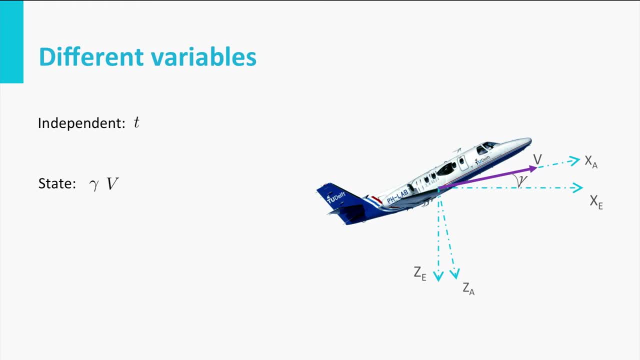 we try to answer questions like how steep can an aircraft climb. Finally, there are several other parameters like thrust, weight, the aerodynamic force, 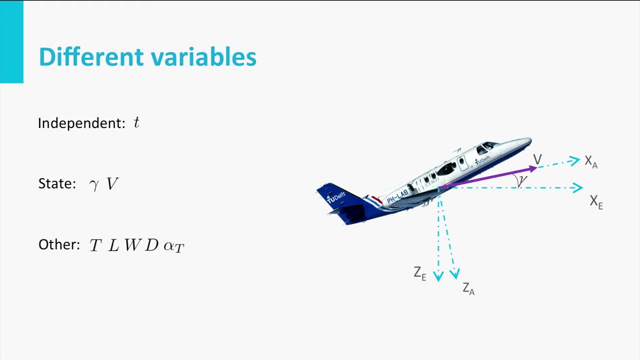 lift and drag, and the angle of attack of the thrust factor. These are all consequential variables. These are all consequential variables. These are all consequential variables. 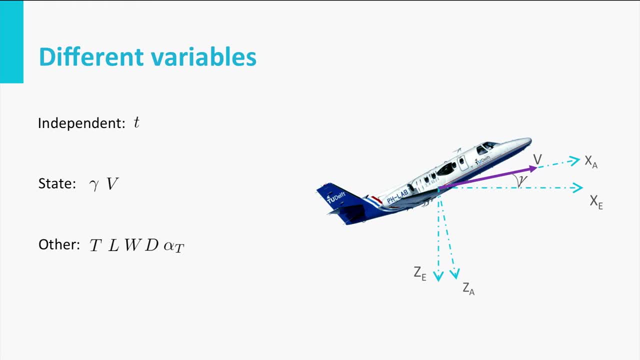 Now, if we can express variables like the aerodynamic force as a function of the state 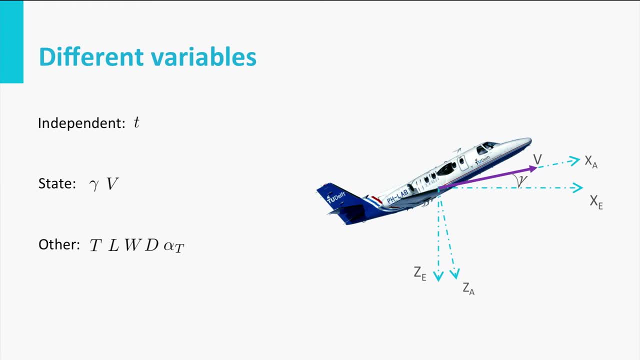 variables v and gamma, then the equations of motion become much simpler. You essentially remove a variable. 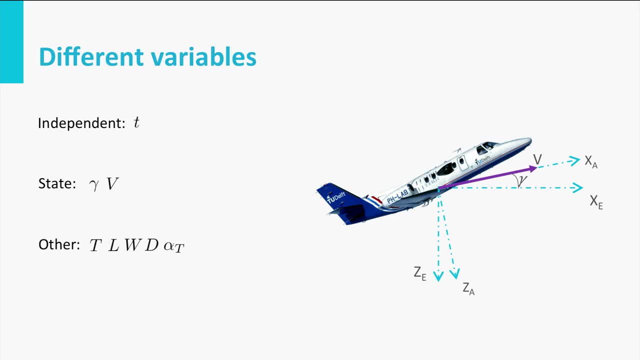 So let's start with the aerodynamic force and try to express it as a function of speed. In the lectures on aerodynamics you have had previously, you learned that the aerodynamic force of a wing can be expressed in the form of a single equation, the lift-drag polar. 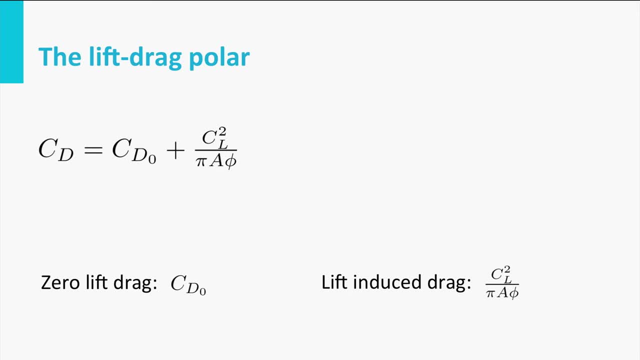 This equation tells us that the drag coefficient consists of two elements, a lift-independent part, zero-lift drag, and a lift-dependent part, the induced drag. 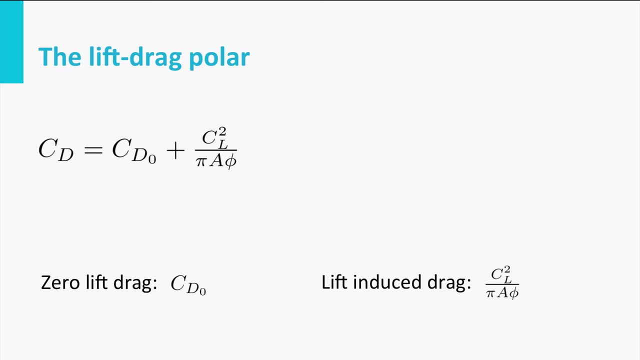 So even when there is no lift, there will be some drag, such as friction drag. This is essentially the same as when you are riding a bike. 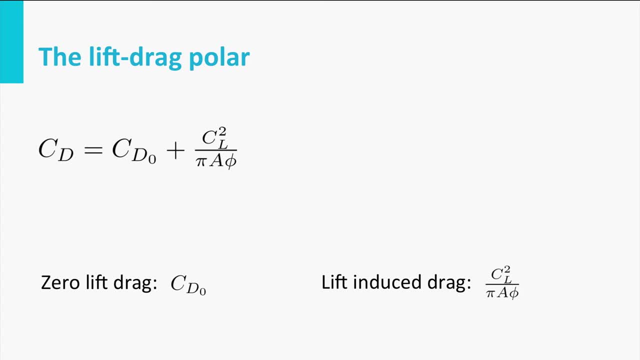 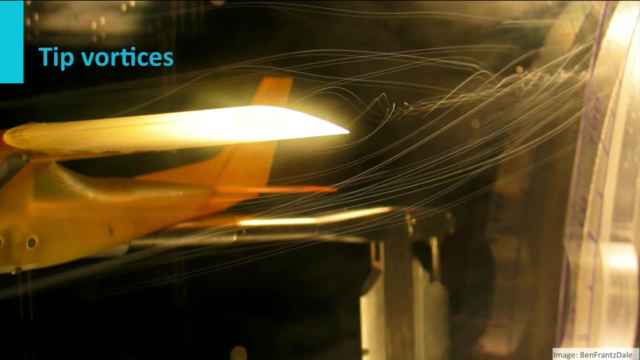 You do not generate aerodynamic lift, but you do experience aerodynamic drag. When a three-dimensional finite wing generates lift, something interesting appears, tip vortices. 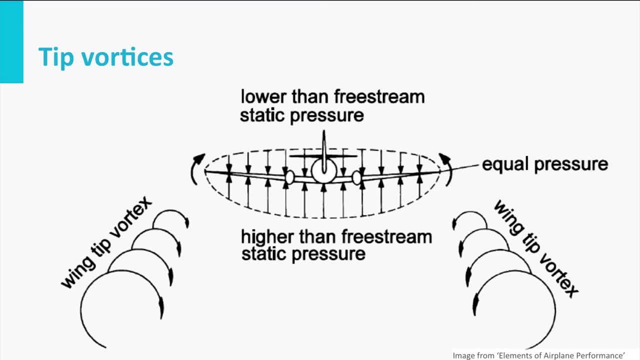 Due to the pressure difference between the upper part of the wing and the lower part of the wing, air will start to flow around the tips in a circular motion, creating wing-tip vortices. 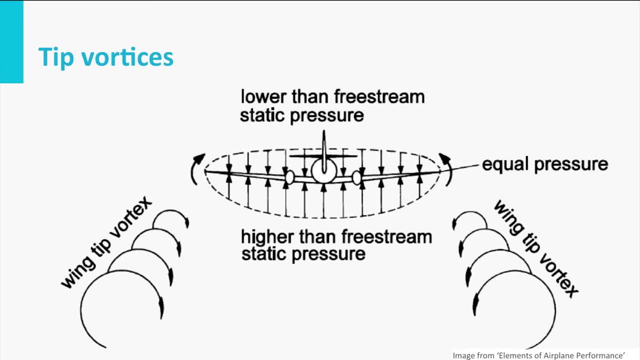 So when an aircraft flies past, it leaves tip vortices in the air. 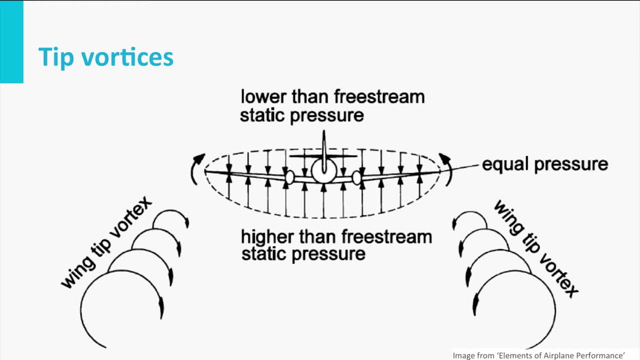 You can imagine that these vortices contain kinetic energy. 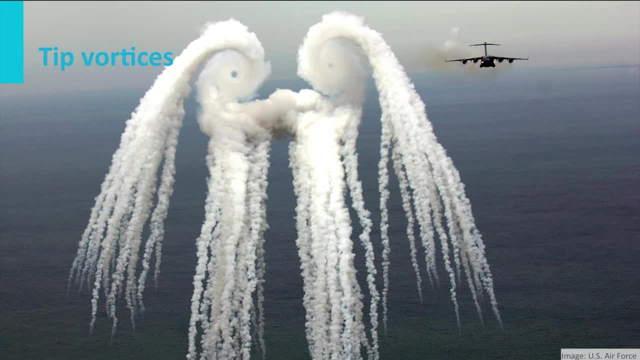 This is essential. This is essentially the cause of aerodynamic drag. 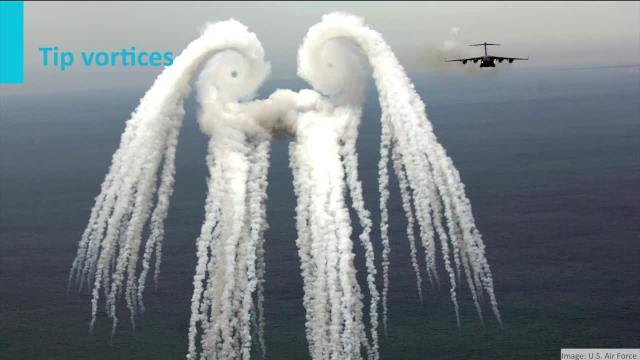 In a two-dimensional case, no tip vortices are left behind, and thus there is no lift-induced drag. 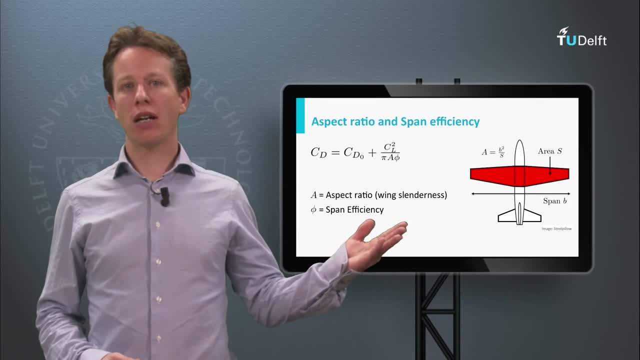 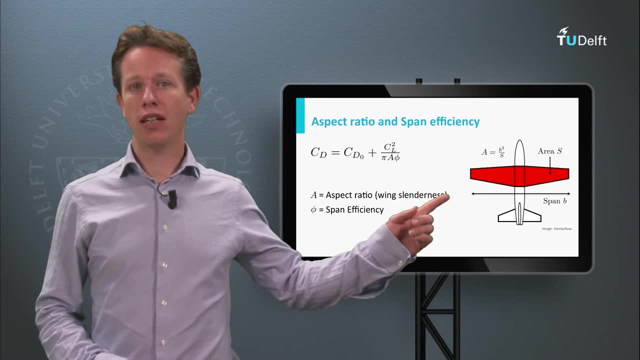 Let's have a look at the equation that relates lift to drag, the lift-drag polar. The parameter a in this equation, aspect ratio, describes how slender the wing is, as indicated by the figure. 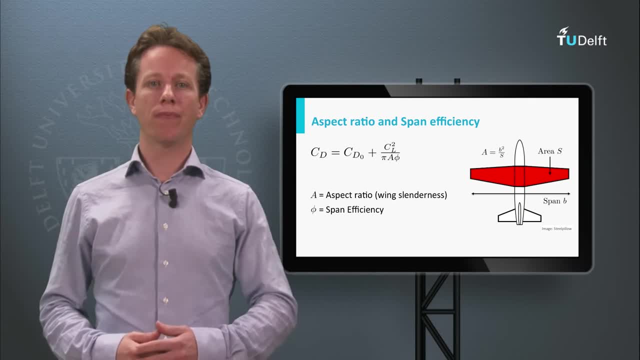 The larger it is, the more the wing approaches a two-dimensional wing. 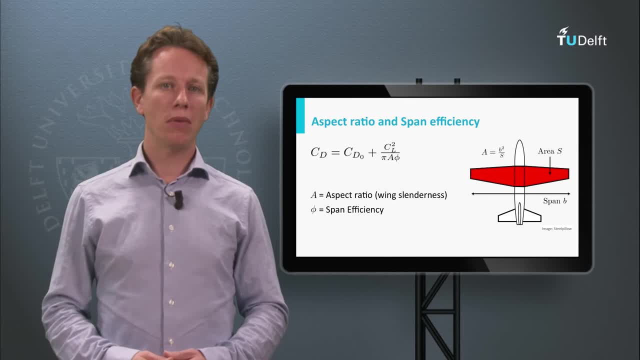 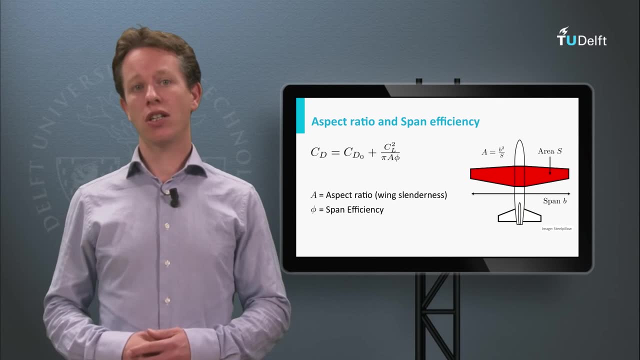 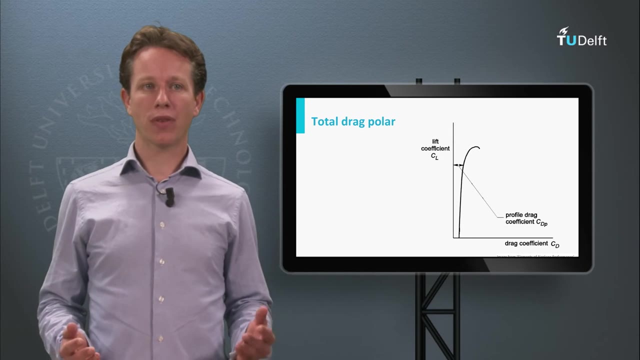 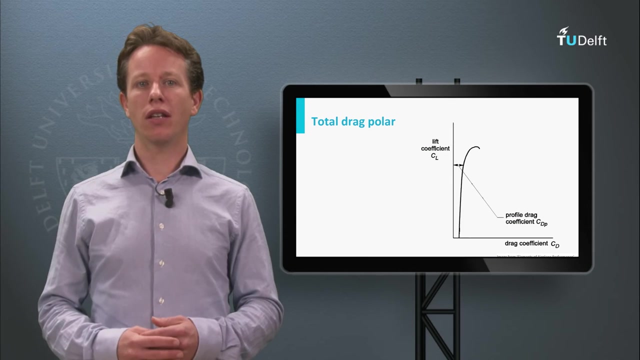 The parameter phi in the equation is the span of the wing. This is the span efficiency, a measure for the lift distribution over the wing. In the ideal case, when the designers have done an excellent job, it actually equals 1. In the current lecture we are not interested in merely the drag of a two-dimensional wing, as indicated in this figure, but in a complete aircraft. The wing by itself is in fact three-dimensional and therefore has lift-induced drag, as represented in the figure. 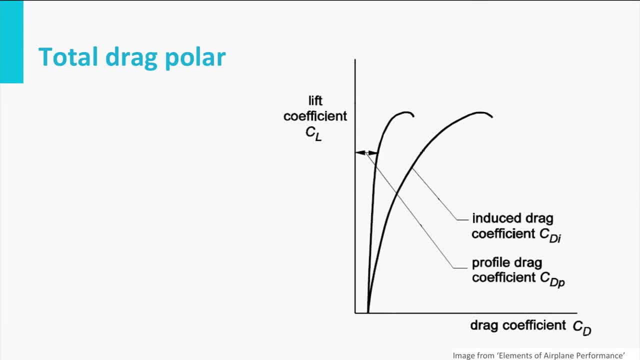 All the other parts of the aircraft, such as the fuselage, the wing, the wing-tip vortices, the fuselage, antennas, vertical stabilizer, also create lift in drag, which we call parasite 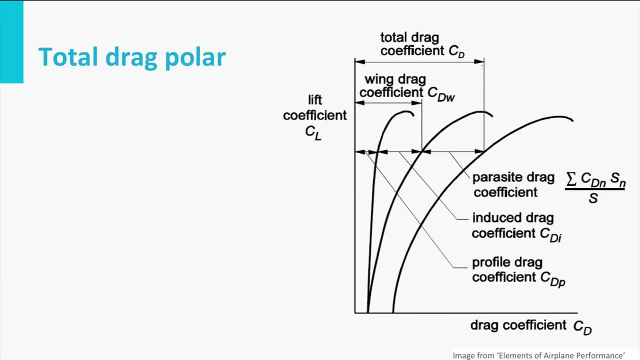 For example, if the fuselage is placed at a zero angle with respect to the flow, it will have a certain amount of drag. 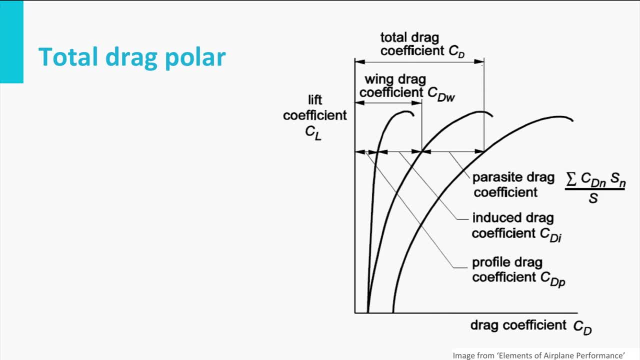 Furthermore, this drag will change if we place the fuselage under an angle. 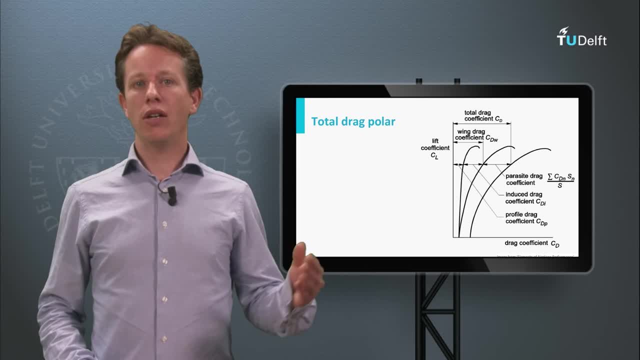 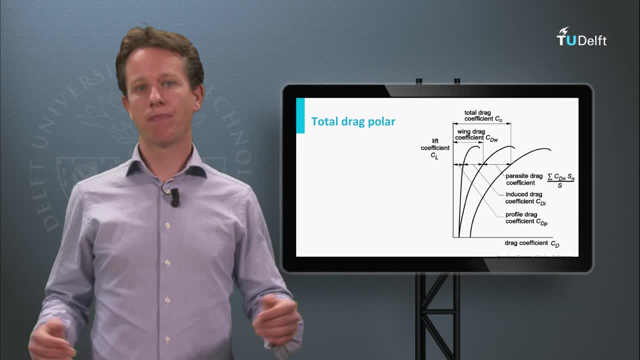 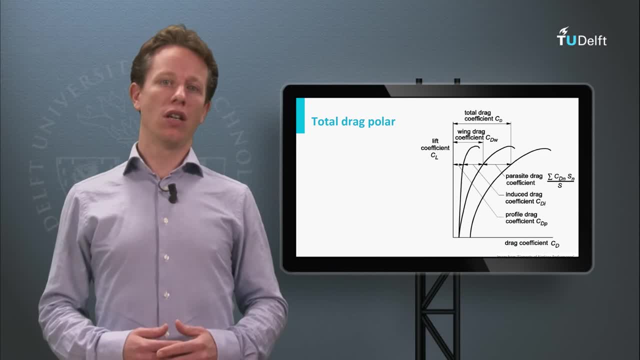 In other words, if we add all these effects to our lift-drag polar, it will mainly shift to the right. 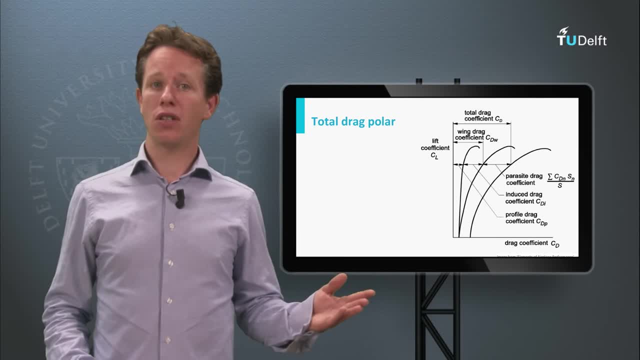 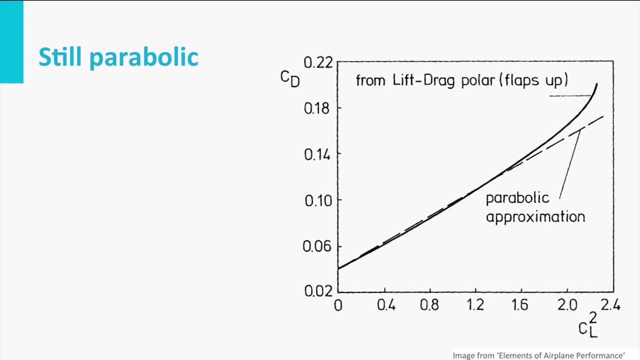 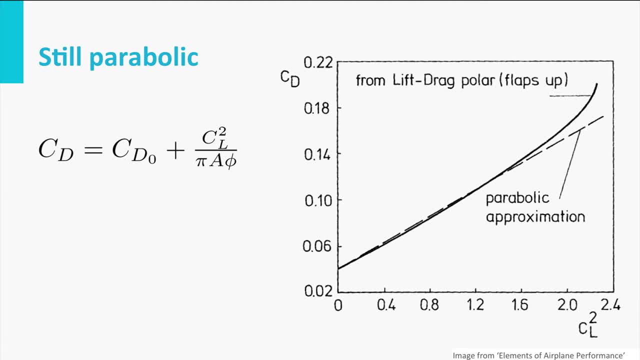 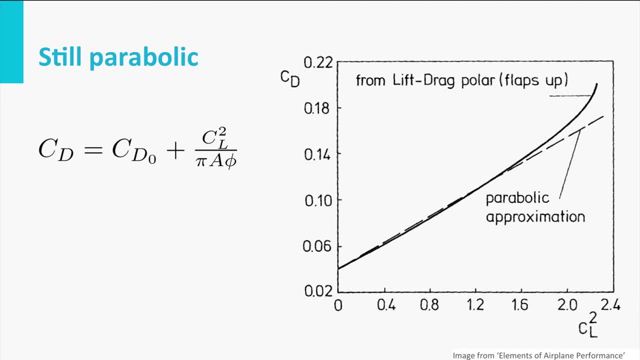 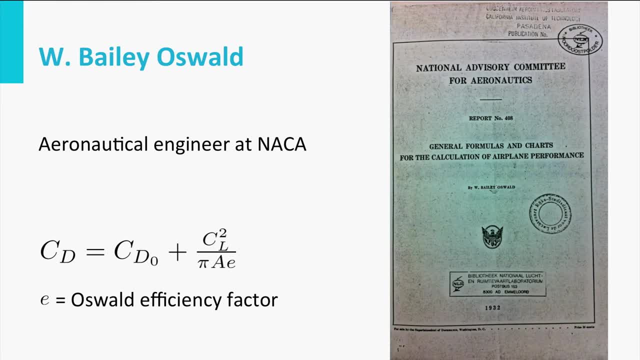 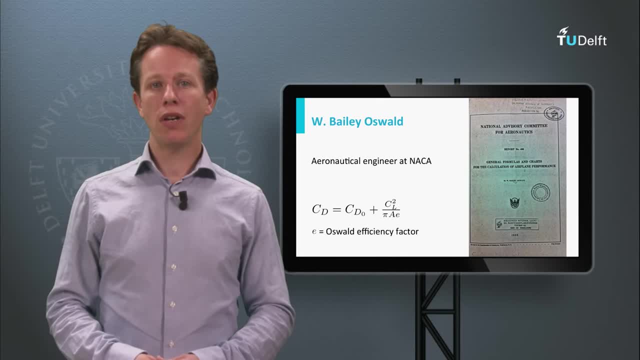 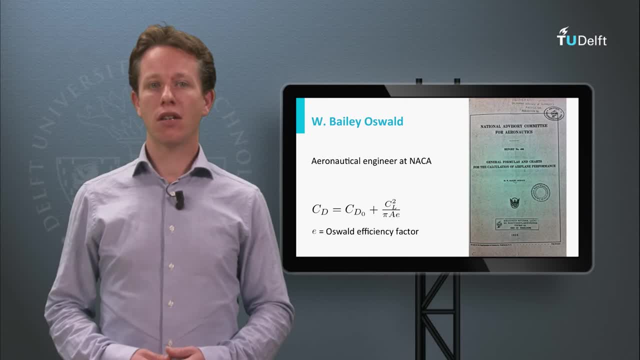 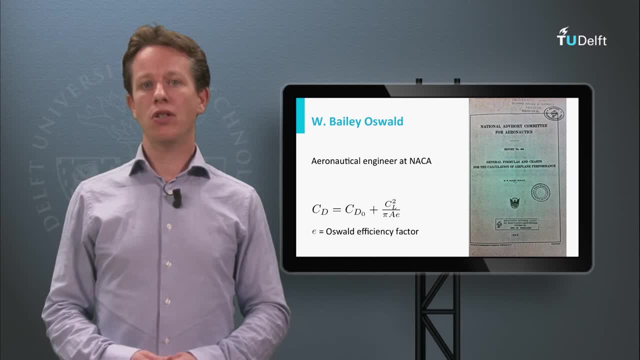 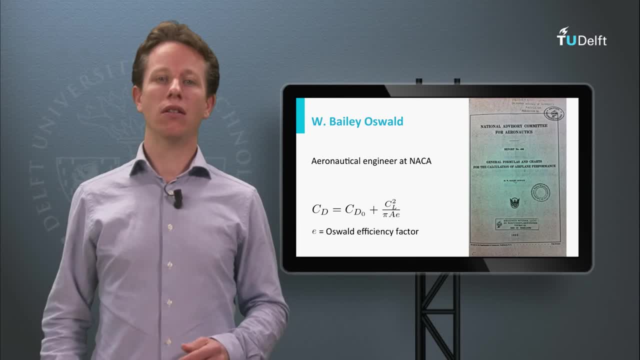 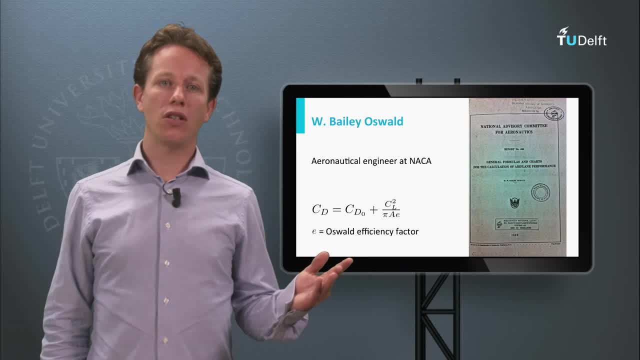 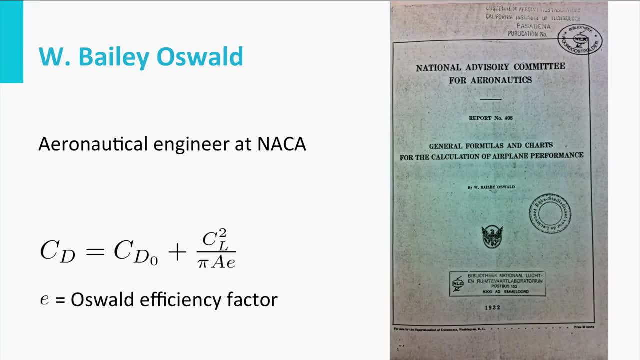 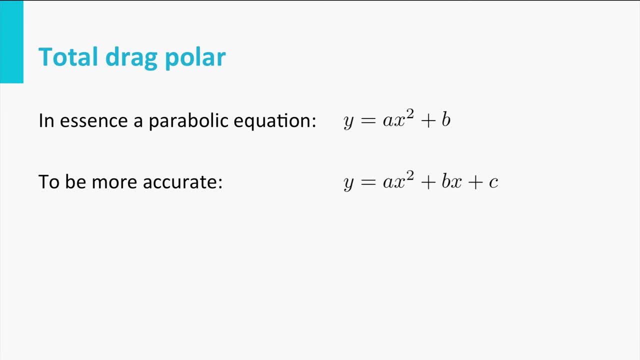 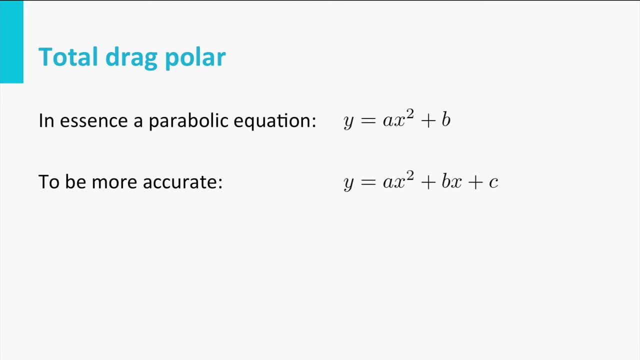 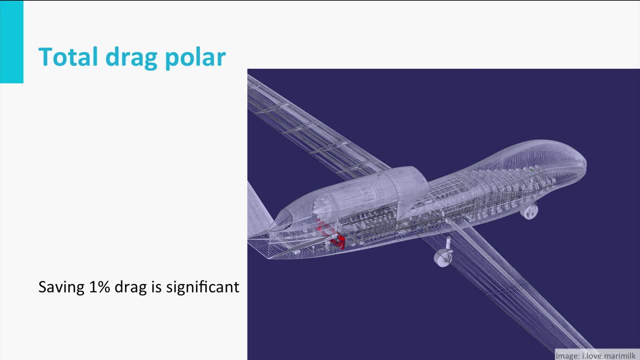 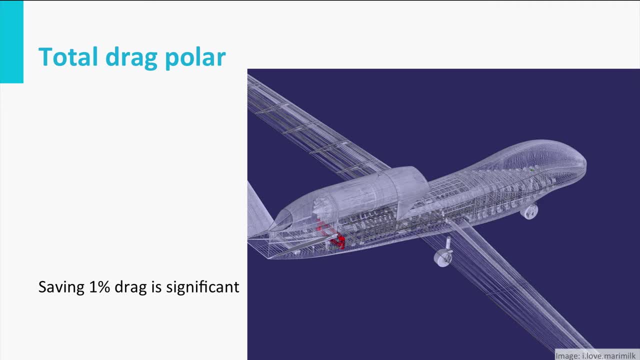 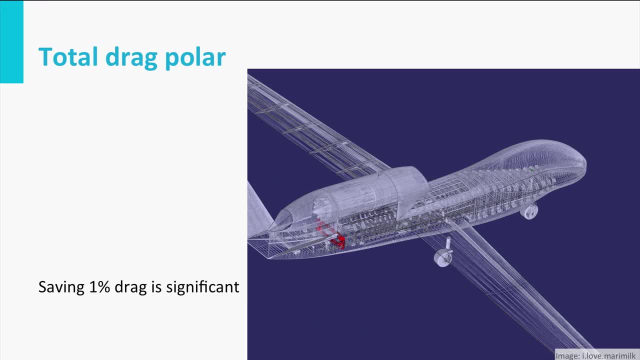 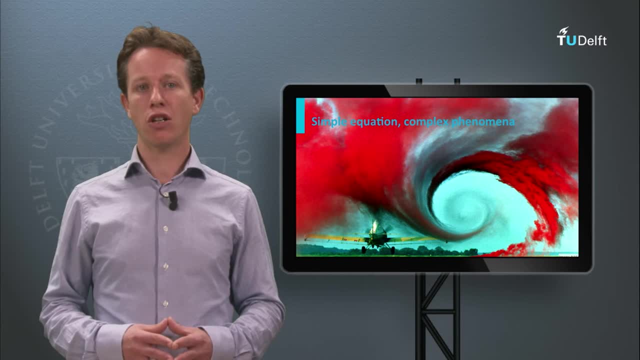 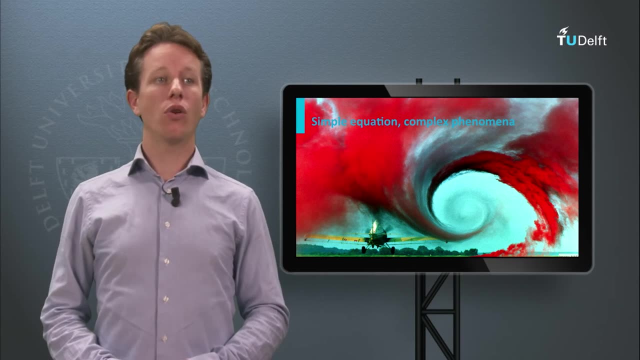 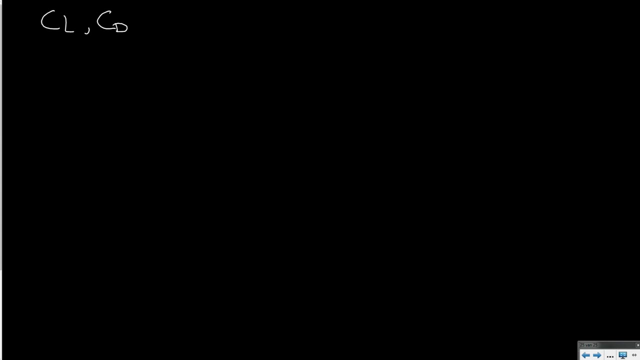 We would like to describe the aerodynamic forces as a function of airspeed in order to simplify the equations of motion. So the lift-drag polar does not give us forces, but coefficients. Ok, so we would like to express actually not the aerodynamics in terms of Cl and Cd but in terms of actual forces. Lift and drag. 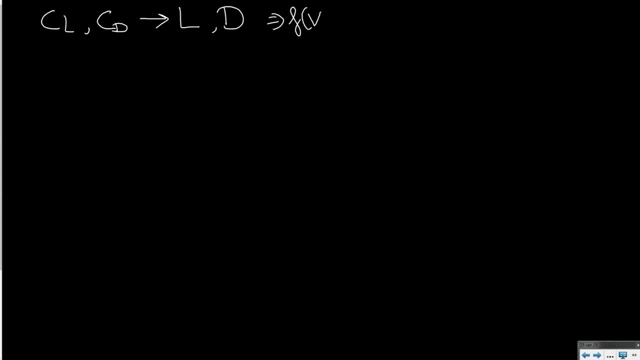 as a function of airspeed, in order to simplify the equations of motion. 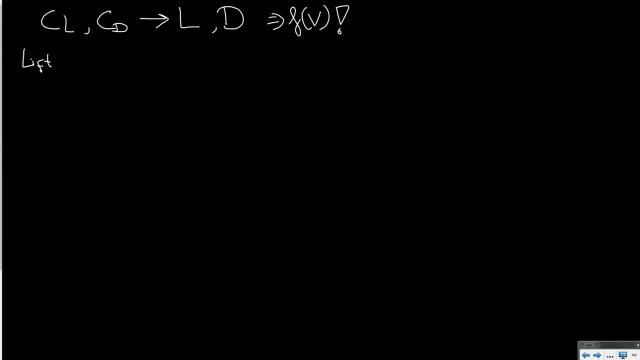 So let us start with lift. We have lift is equal to weight and if we write out this equation, then we obtain CL times a half rho V squared S is equal to the weight. 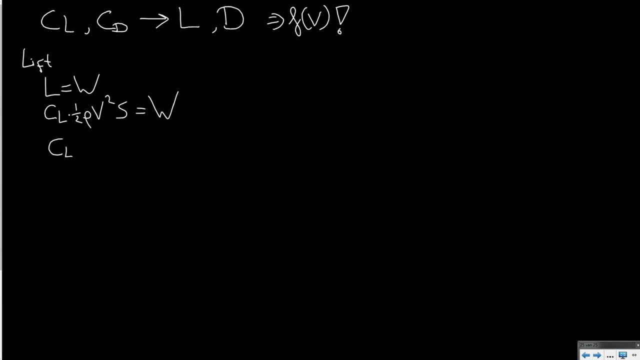 So in other words we can also bring CL to the left hand side of the equation and state that this should be equal to weight divided by S, 2 over rho and 1 over V squared. Now on the other hand. 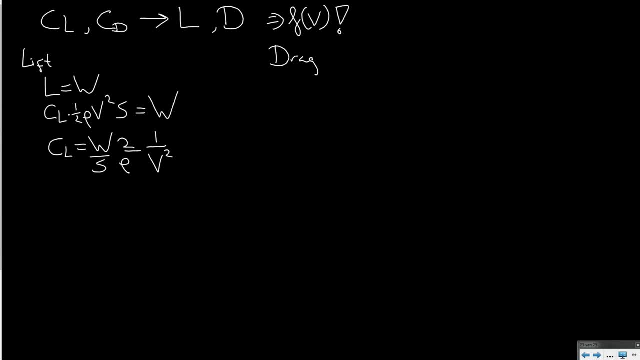 We also have drag. And let us express what the drag of an aircraft is starting with the parabolic lift drag polar. So we have CD, CD0 plus K1 times CL plus K2 times CL squared. Now this is only the drag coefficient. And we should write it out. In order to obtain the actual drag. 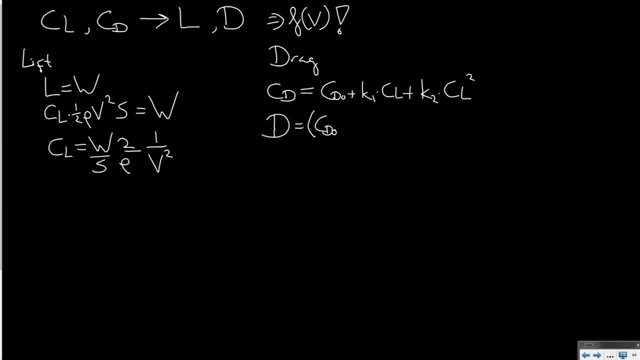 So the actual drag is the drag coefficient CD0 plus K1 times CL plus K2 times CL squared multiplied with the dynamic pressure half rho V squared and the wing surface area of the aircraft. So interestingly. We now have. 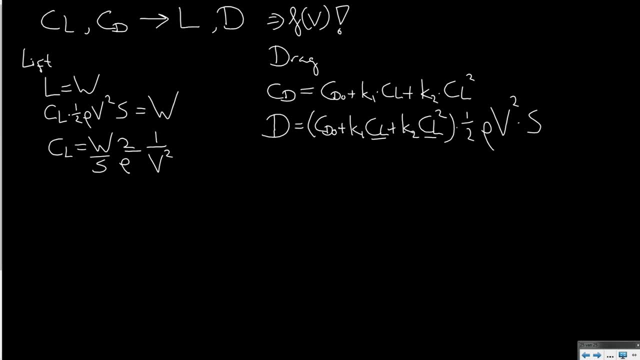 We now have CL over here in the equation and the other factors CD0, K2, half rho and S are constant. And finally we have airspeed which is nice because we would like to have aerodynamic drag as a function of airspeed. So we have one simple problem. 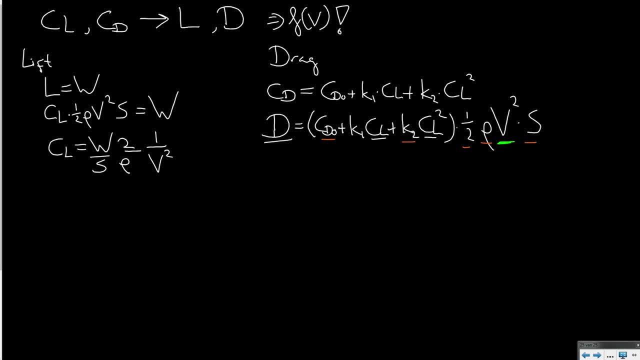 We have one equation with two unknowns CL and V. But. As you see. 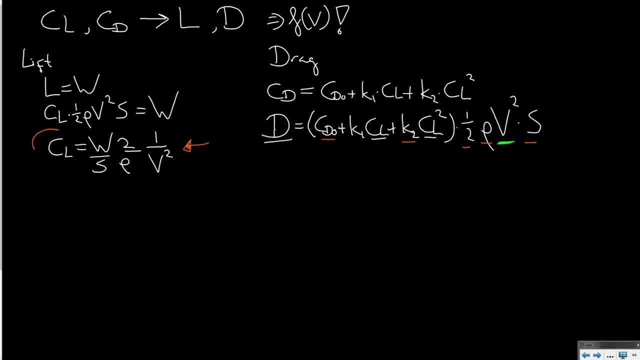 On the left hand side here. We can actually express CL as a function of airspeed. 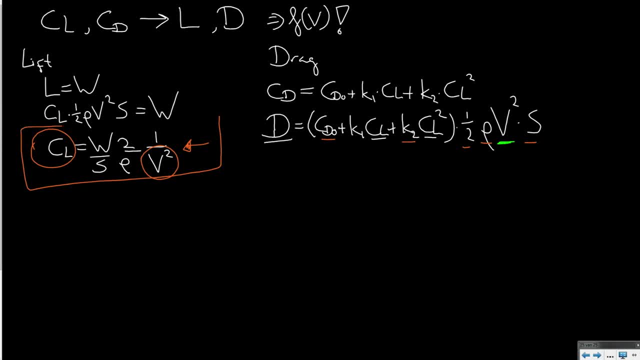 So let us insert this whole equation in the drag equation. If we do that. 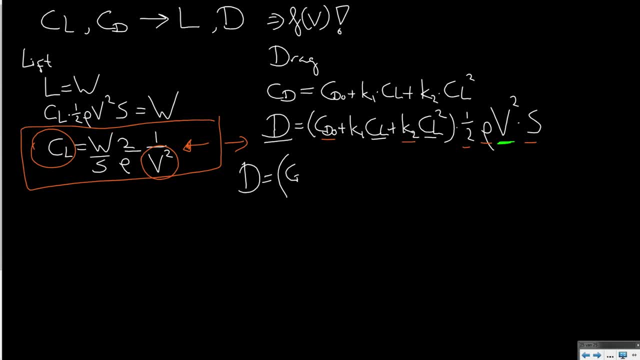 We can state that drag is still CD0. 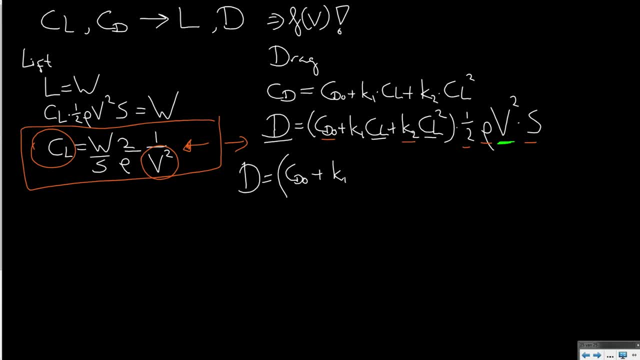 Plus. K1 times. CL and that is weight over S, two over rho and one over V squared plus K2 times the same equation one over V squared. This whole thing squared. And all of this. Has to be multiplied. With a half rho V squared S. So it is starting to become quite a long and lengthy equation. 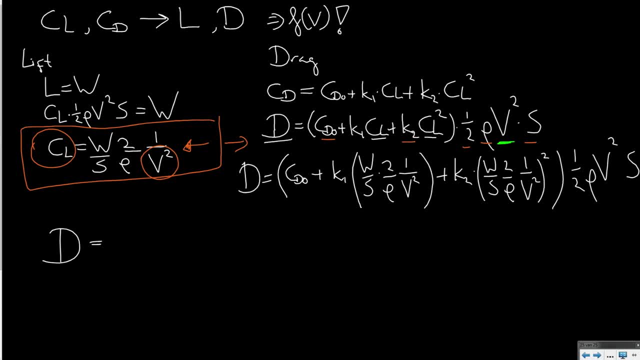 But let us just see what it looks like and try to interpret what it means. It basically means I have. 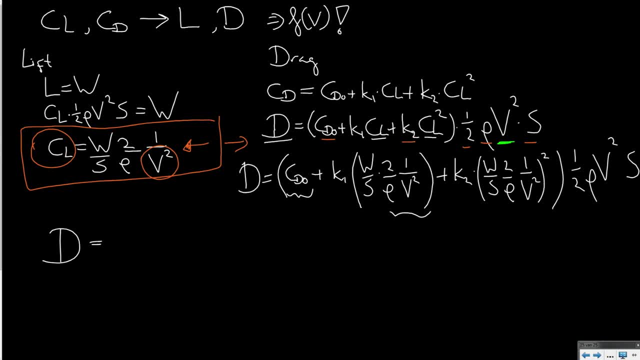 If I take all the elements separately. I have drag is equal to CD0. 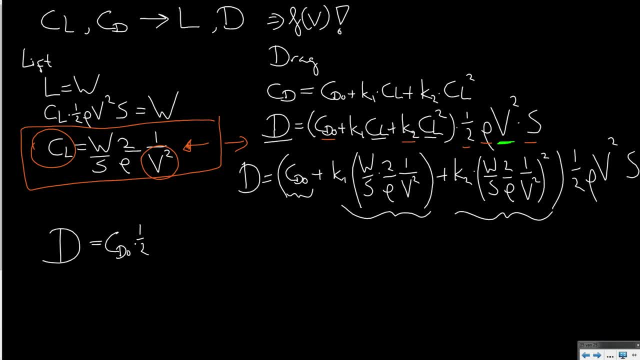 Times a half rho V squared S. Plus K1 times weight over S, two over rho, one over V squared. Multiplied with a half rho V squared S. And I have drag is equal to CD0 times a half rho V squared S. Plus K1 times weight over S, two over rho, one over V squared. Multiplied with a half rho V squared S. And I have drag is equal to CD0. 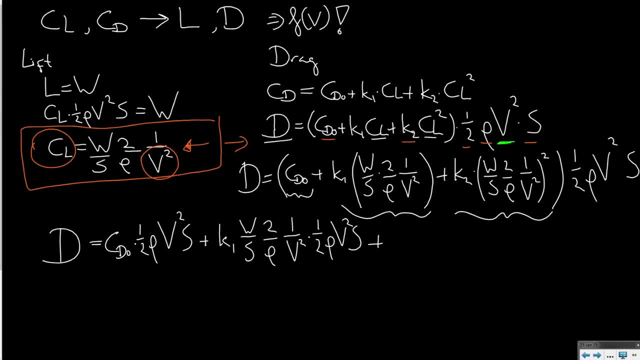 Plus K1 times weight over S, two over rho, one over V squared. Multiplied with a half rho V squared S. So a long equation but we can actually remove some terms in the equation. 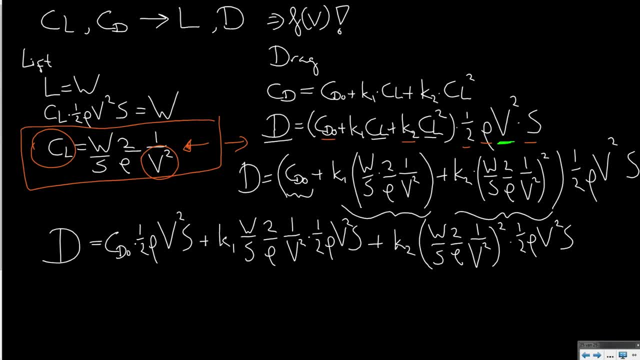 So a long equation but we can actually remove some terms in the equation. So a long equation. 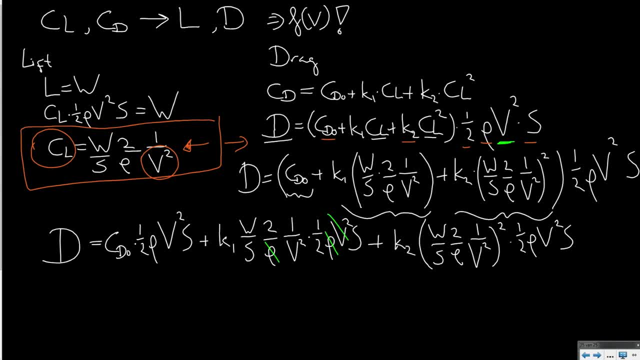 Clearly we see a row here and a row there, we see a v-square there and a v-square there, a 2 and a 2 and an s and an s. 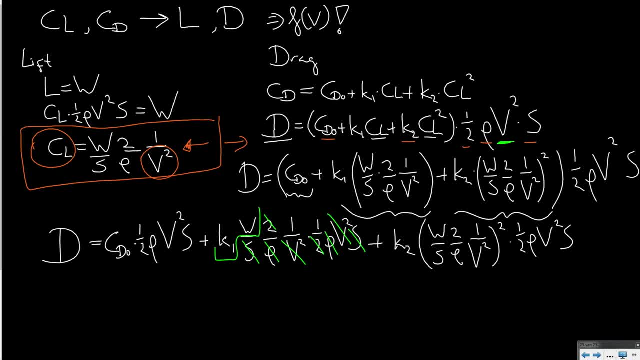 So the only thing that remains of this part is k1 times w. 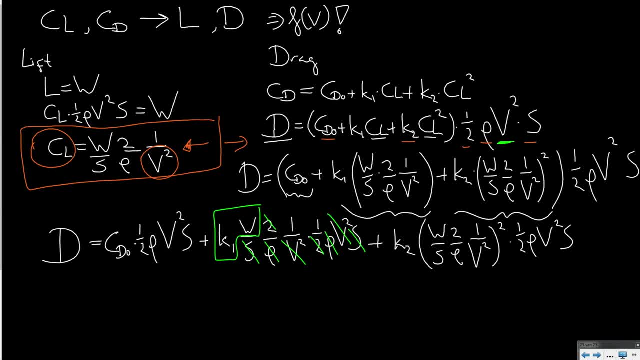 On the other hand we have this lengthy equation and you can actually see that over here we have v-squared squared, which is essentially v to the power 4 and we also have a v-squared over here. 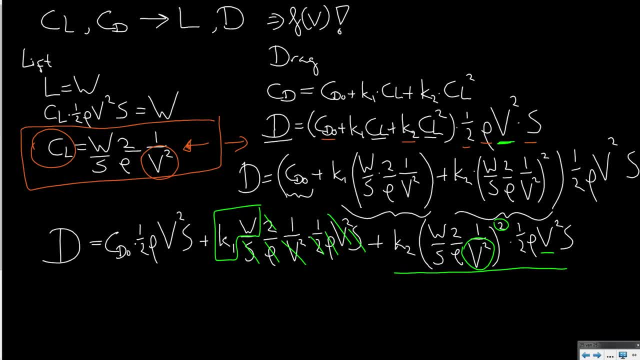 So let us write what we now have in a slightly more simplified form. We have drag cd0 half row v-squared s and we have a v-squared over here and a v-squared over here. So let us write what we now have in a slightly more simplified form. We have k1 times w and if I write out the final term I will actually obtain k2 times weight squared from here. 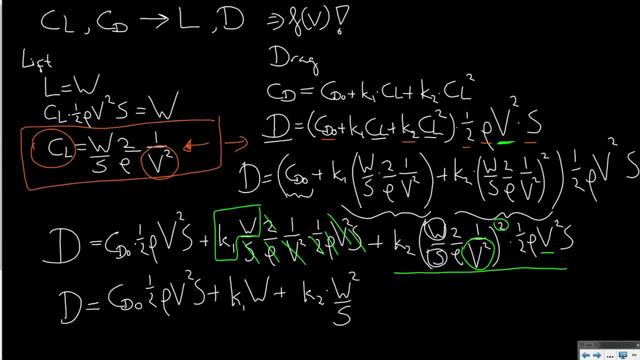 I am left with one wing surface area because I have one over here as well. 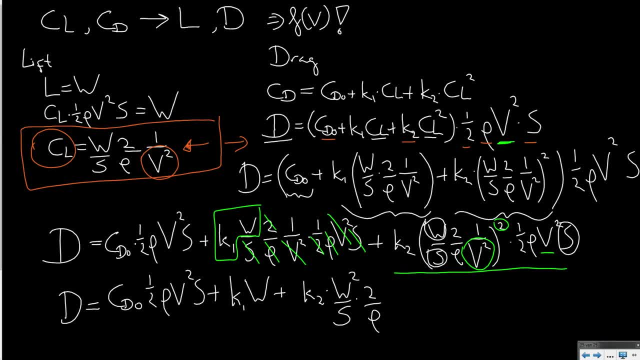 I am left with 2 divided by the air density and I am left with 1 over v-squared. 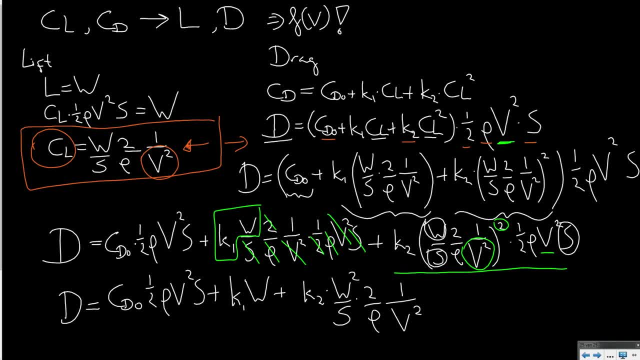 And essentially I now have a part of zero lift drag and I basically also have lift induced drag on the right hand side. 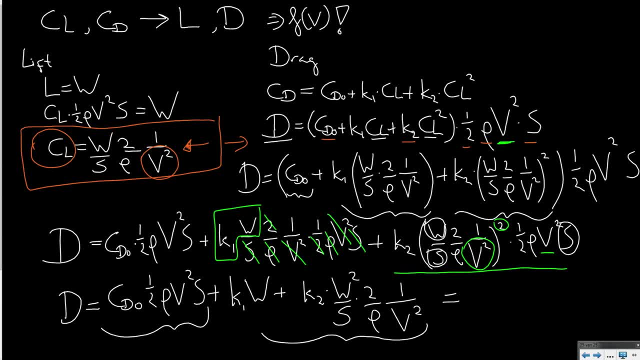 But now have a look at this equation. A bit more carefully because if you look at all the terms cd0 is constant, half is constant, we are considering one air density, a specific altitude, s wing surface area is constant, we are considering one aircraft with a given weight, k2 is constant, this weight is constant, s is constant, still at a constant altitude. So essentially we have a, 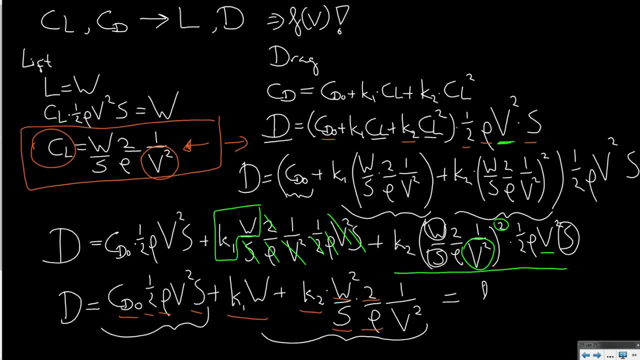 a function of v-squared plus a function of 1 over v-squared. And this shows us how drag is related to airspeed.